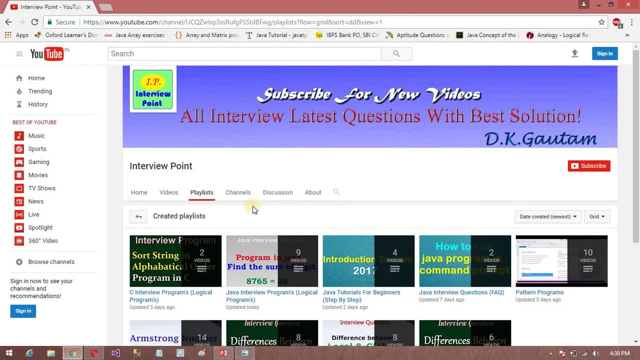 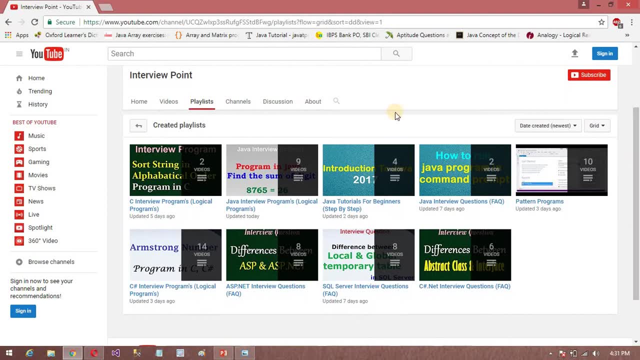 if you till now did not subscribe my YouTube channel, then please subscribe my YouTube channel If you want. Here you will get all the most important interview questions, latest interview questions, C interview questions and Java interview program, Java tutorials for beginners and Java interview point. 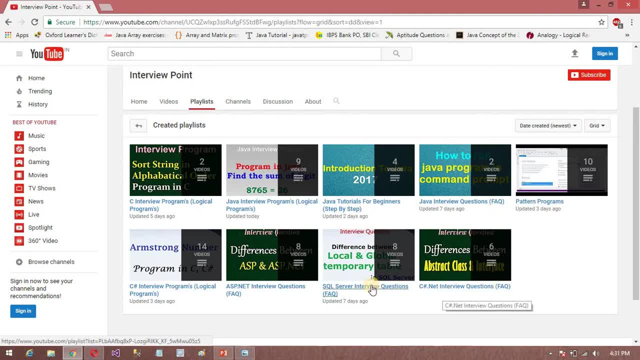 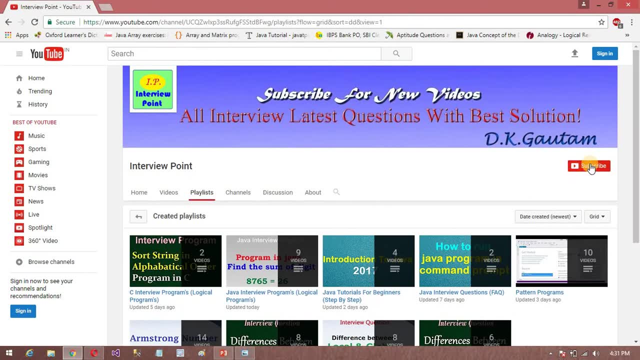 Interview questions. tracking programs: C sub-interview questions, SQL server, ASPNET and CISAS. So here you will get all the latest interview questions, So don't forget to subscribe my YouTube channel interview panel. So now let's start the program. 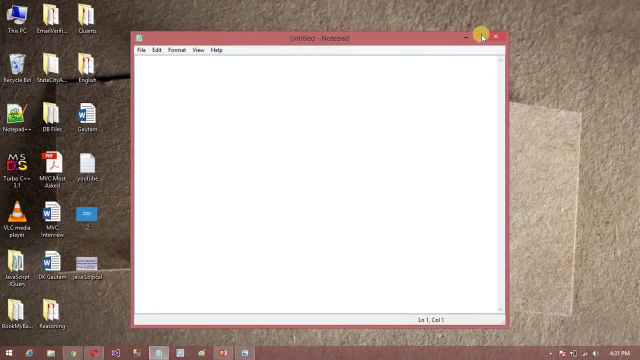 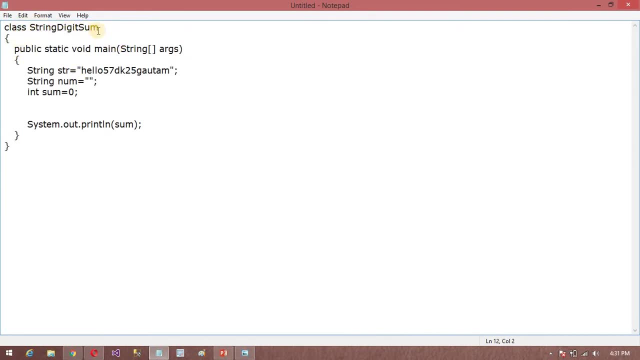 I am going to open my notepad Here. I have tab forum, So here class string digit sum. Ok, my class name is string digit sum, So I have created this main method here And string is method. You can also give it as dynamic. 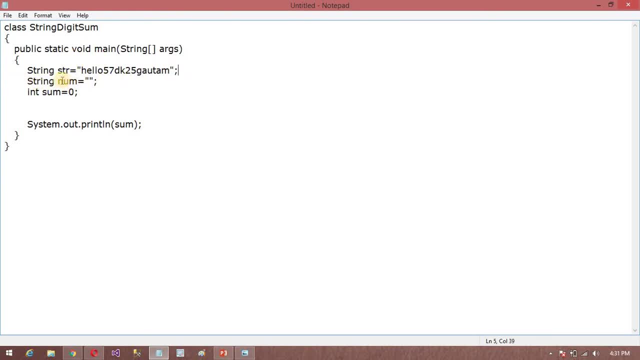 So no problem. And string: I have created bug mode variable here. none, So it is now empty. Ingestion variable for addition purpose: Ok, So you have to find out the sum of this: 57 or 25.. 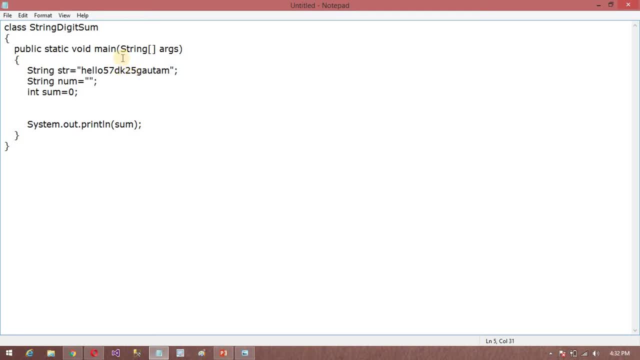 Doesn't matter, You can have any other number in here, Ok, But it is the example. So I am going to show you the logic of this program. So first we will do for loop. So in this for loop, 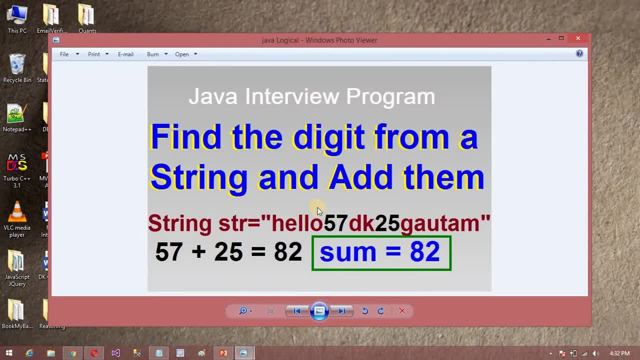 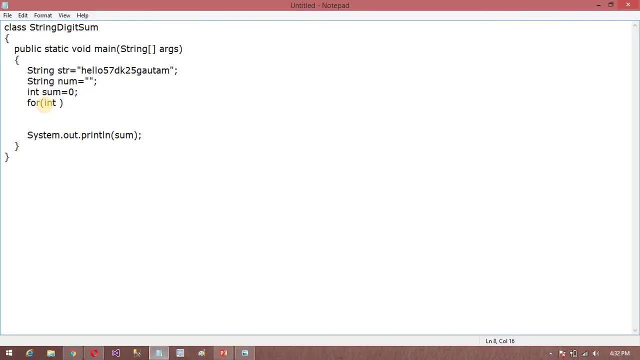 Now program is: I want to find out the digit sum. Ok, This digit sum, Ok. So now can I write the program. So now start it First. i is equal to 0. So i less than extra is nothing, nothing. 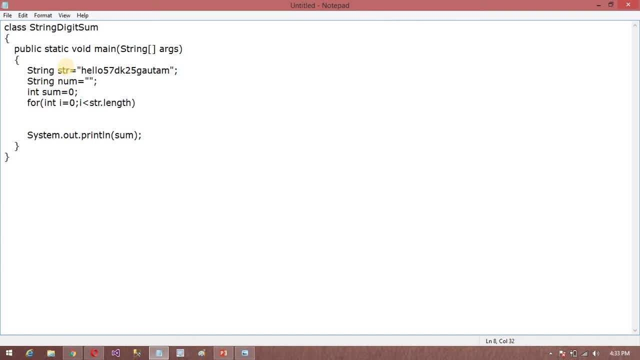 This is string for, Then i plus Ok After that. what I want to do here In this loop, I want to write condition. So if character dot, each digit, is digit, Then string means String means str, dot, care act. 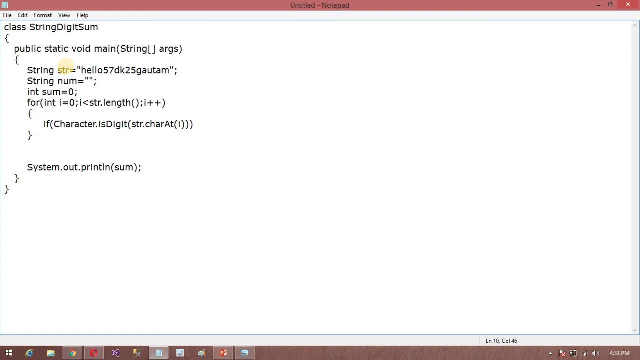 Act is nothing, but i- Ok, Be carefully, guys- The most important program, But most of the candidates are not able to do this, So some of my students gives me this program, So num is equal to What I want to do here. 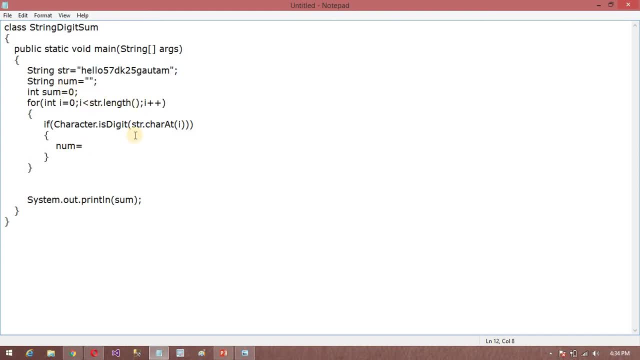 I want to add this value, This loop, if we will find out this number, So it will add in this num variable. Ok, So num is equal to num plus str. dot. care act. Ok, Care act is nothing but i. 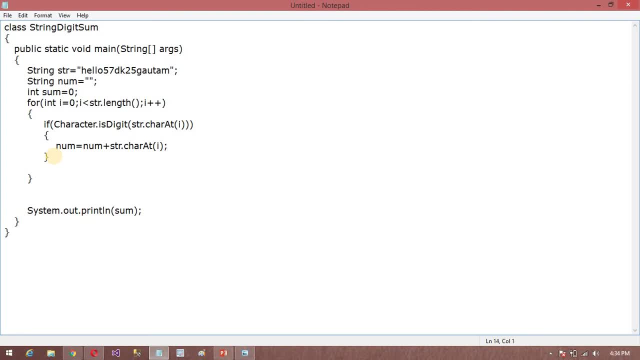 Ok. So after that, What I want to do here In the else condition- Else condition- I want to write: If num dot equals Equals empty, Ok, Then sum is equal to sum plus integer, integer dot parts and int. 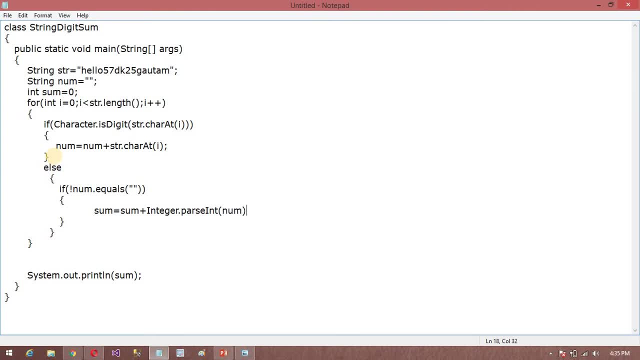 Number. I want to pass the number. Ok, we pass here. You can see, here the number will be the same. Ok, after that I want to empty this number here. So for that purpose, number is equal to n. 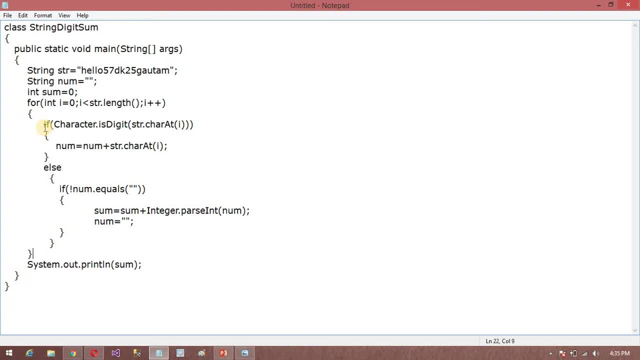 Ok, in the end of this rule I want to print this sum. Ok, let's first understand the logic of this theorem. Ok, So now understand the logic. So it will start from 0 to string of length. Ok, 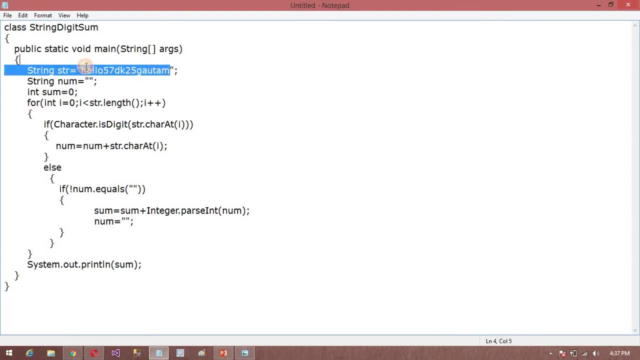 0 is nothing but h value and length. It is above string length 1,, 2,, 3,, 4,, 5,, 6,, 7,, 8,, 9,, 10,, 11,, 12,, 13,, 14,, 15,, 16,, 17.. 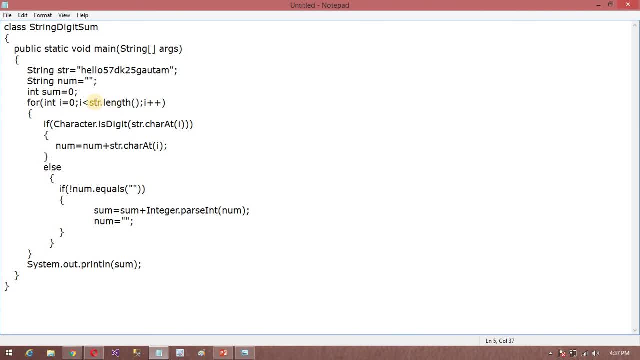 String length is 17. So it will execute till this condition is true, So suppose It will reach at 5 position. That means the 5 index string is deleted, So it will end 5.. Ok, So after that what it will do. 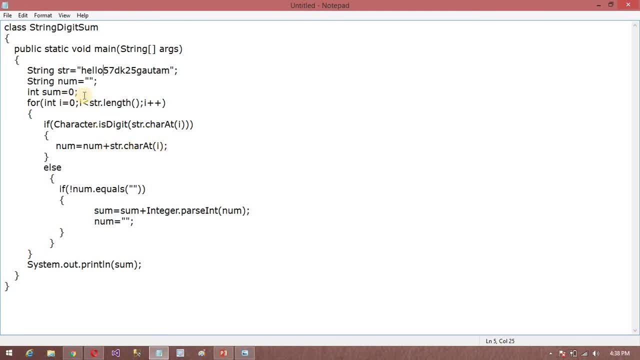 num is equal to num plus string of char at i. So this char at i is nothing but the position of this index. index position. Ok, So in the 5 position it will end at 5.. So 5, what it will do. 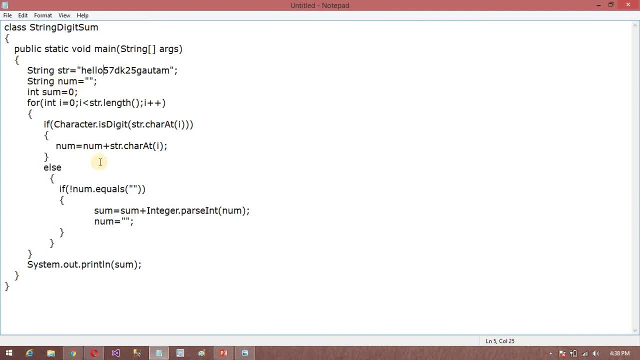 It will add in this string: variable, num variable. Ok, Add as a character. Ok, So it is the string. So after that it will execute till then it will find the character. If not found, then what it will do. 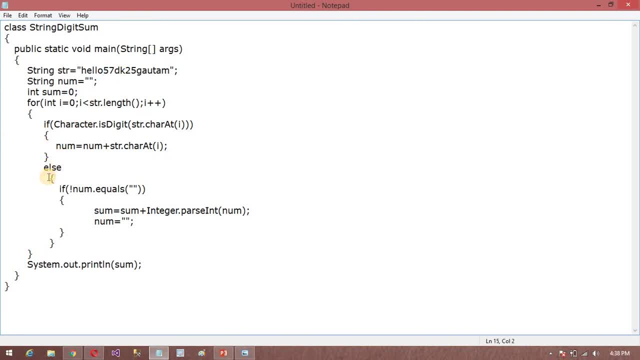 Add in the else part. It will. you can see here in the else part. So in the else part, If num is not equal to, If num is not equal to because this empty, That means here we have a num or more, more numbers. 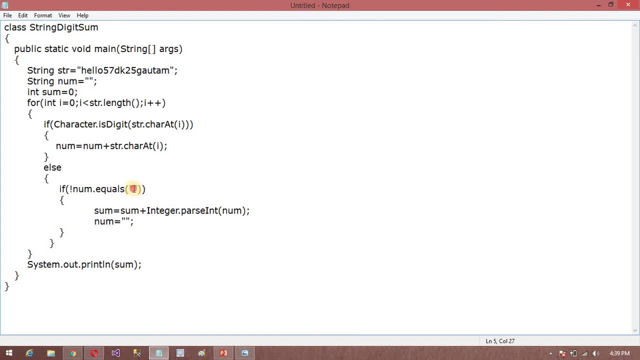 Ok, More characters. So it will, it condition is true. If the condition is true, then it will come here and sum. Sum is nothing but integer variable. So it will add: because it is parsing Why it is parsing. 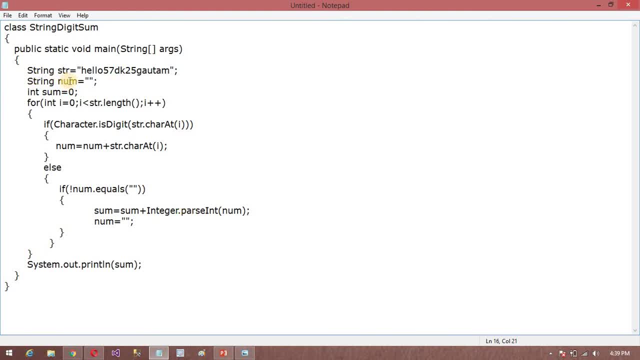 Because here you can see, here it is the string variable. Ok, So we need to parse. Ok, in the integer. that's why I am using integer for parsing. ok, so it will parse, and after that adding this number in some variable. after that it will empty. 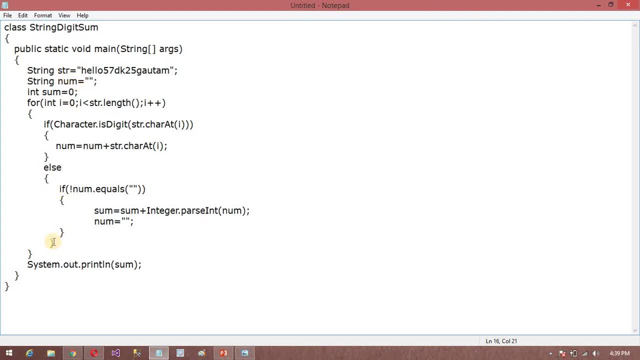 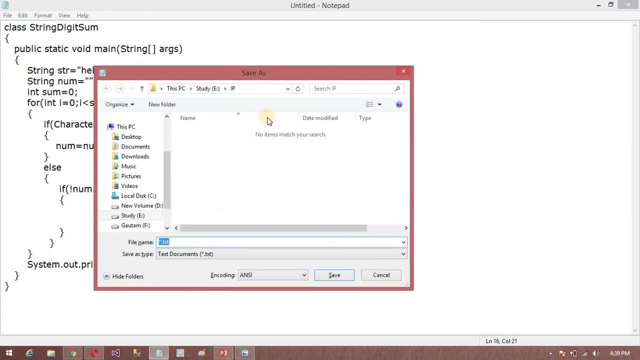 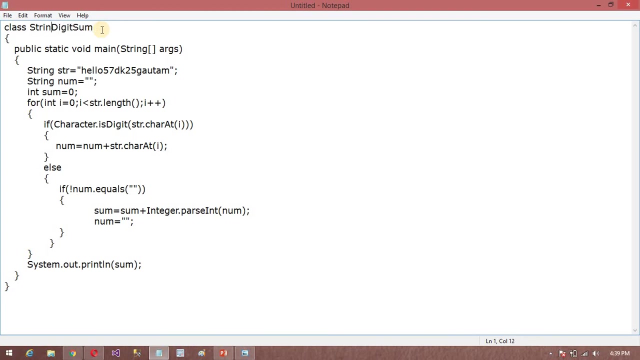 this num variable so it will execute and give you the output to the user. so now I am going to save this torrent. so my class name is string digit sum. so first suppose my class name is nrn. ok, digits, my class name is digit sum.